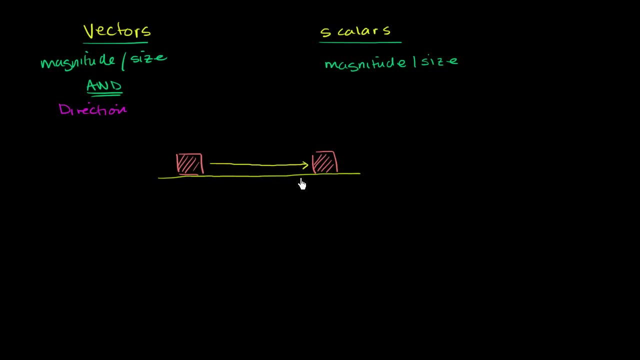 So I move the brick right over there And then I take a ruler out and I say wow, I've moved the brick. I have moved the brick 5 meters. So my question to you is: my measurement of 5 meters is it a vector or a scalar? 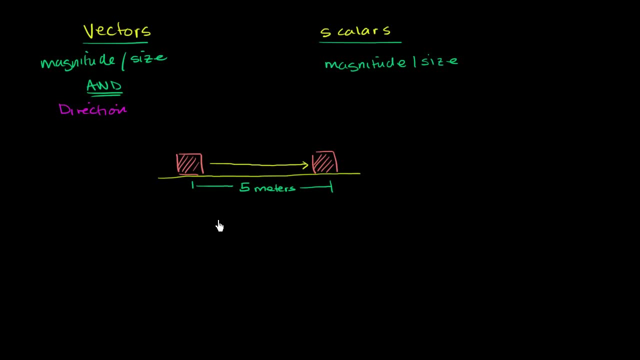 Well, if I just tell you 5 meters, you just know the size of the movement, You just know the magnitude of the movement. So if someone were to just say 5 meters, this is a scalar quantity And when we're referring to moving something, or how much something has, I guess, changed its position. 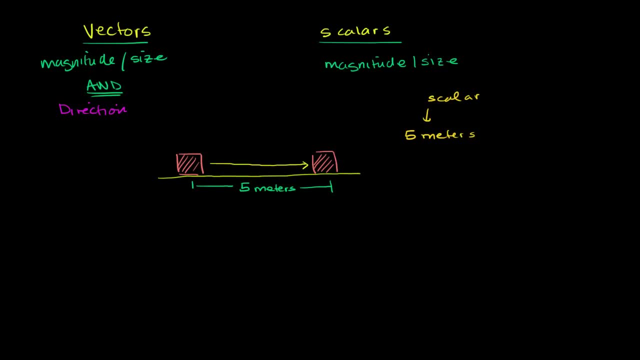 and I don't give you the direction. we're talking about distance, And I'm assuming you've heard the word distance. How far of a distance has something traveled? So this is distance. So we could say that this block or this brick, because of my picking it up and moving it, 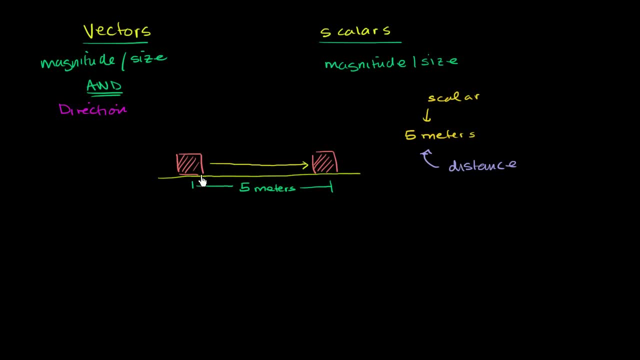 has moved a distance of 5 meters. But if I didn't show you this picture here and someone just told you that it moved a distance of 5 meters, you wouldn't know if it moved to the right 5 meters. you wouldn't know if it moved to the left 5 meters. 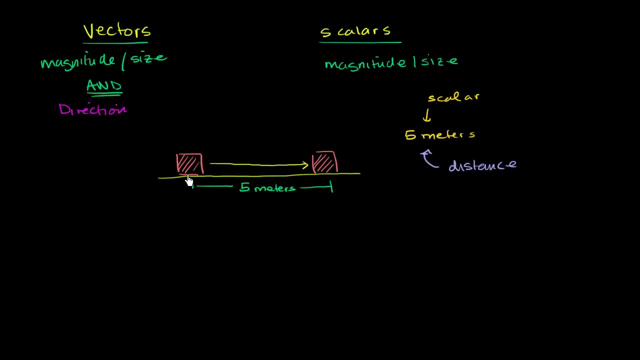 if it moved up or down or in or out, or you don't know what direction it moved. 5 meters. You just know it moved 5 meters. If you want to specify that so we could say that this brick right over here. 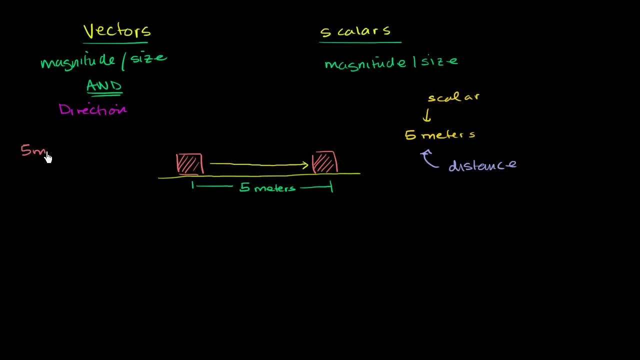 that it moved 5 meters to the left. So now we have specified a magnitude right over there, So that is a magnitude, And we have specified a direction to the left. So you now explicitly know that it went 5 meters to the. 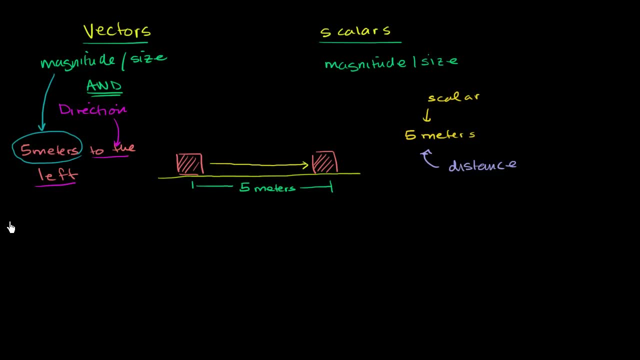 oh sorry, it should be 5 meters to the right. Let me change that. So 5 meters to the right is what it got moved. It started here. it went 5 meters to the right, So once again the magnitude is 5 meters. 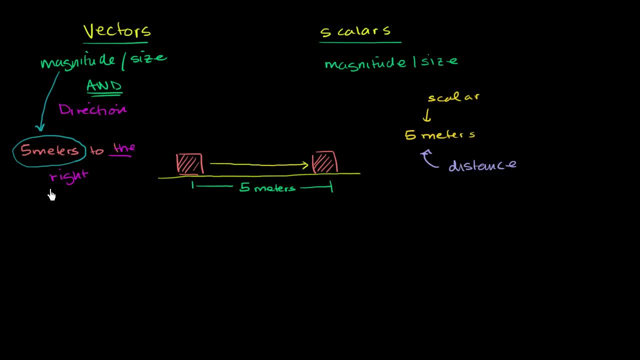 and the direction is to the right. So what I've just described to you right here is a vector quantity. So this, all of this business right over here, this is a vector. And when you talk about the movement, the change in position, 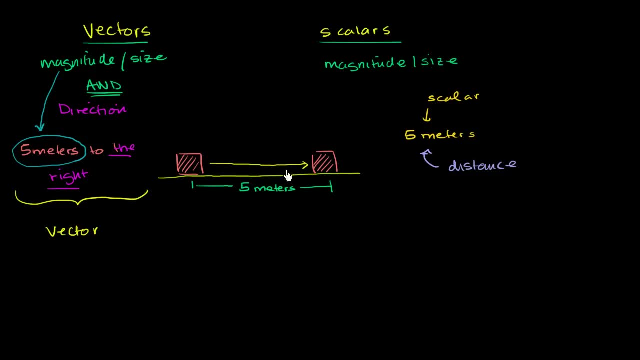 and you give its direction. the vector version of distance, I guess you could call it, is displacement. So this right here is displacement, Displacement. So the correct thing to say you would say that this brick has been displaced 5 meters to the right. 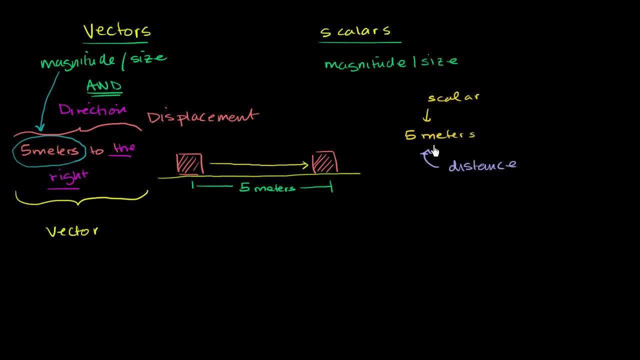 Or it has been moved a distance of 5 meters. Distance is a scalar quantity. I didn't tell you what direction we moved it in. Displacement is a vector quantity. We told you that it is to the right. Now let's explore this. if we talk about the actual, 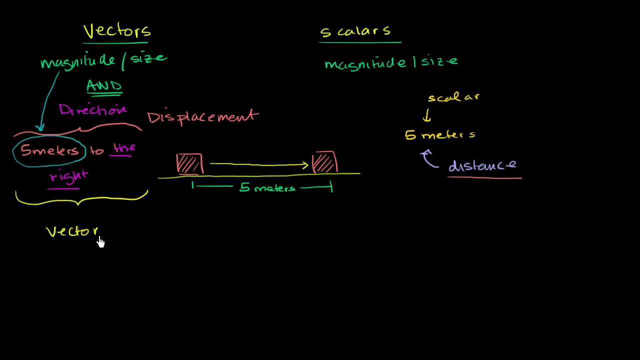 well, we'll talk about the speed or velocity of something. So let's say that my, let's say that my, that this 5 meters was traveled, and let's say that the change in time, let's say that the change in time. 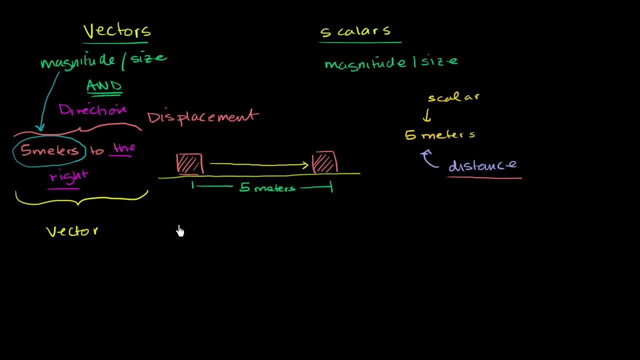 and when I let me, just because you're probably not familiar with what that means. So let's say that the change in time right here change in time when I moved this block 5 meters, let's say that it was. 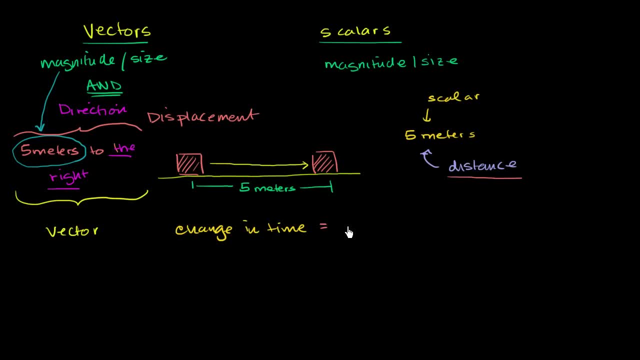 I don't know. let's say that this, the change in time, was 2 seconds, So maybe right when I, when the block started moving, maybe on my stopwatch it said 0, and then on my stopwatch when it stopped moving. 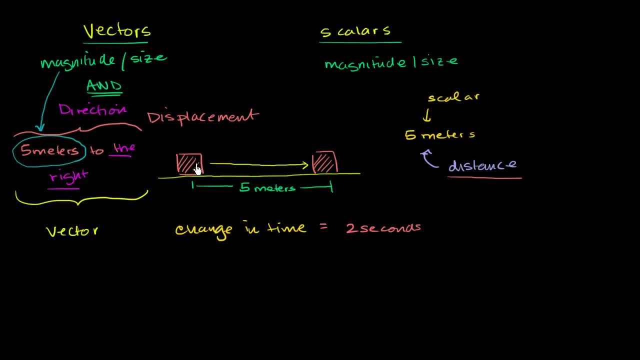 it said, or when it got to this position. I should say, when it left from this position, my stopwatch said 0,. when it got to this position, my stopwatch said 2 seconds. So the change in time or the duration we're dealing with, 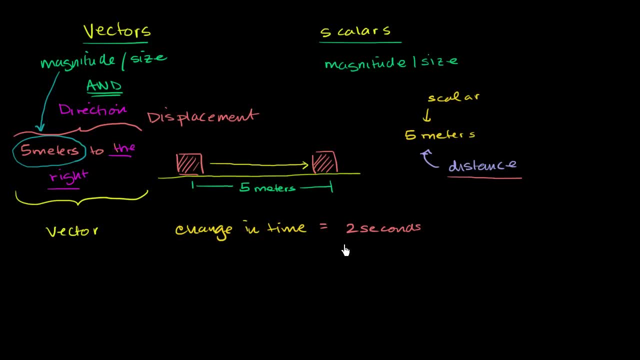 is 2 seconds And this is you know, for all we know, time only goes in the positive direction. So you could, you know, you could assume that it's well, you could, you could pick that as a vector or a scalar quantity. 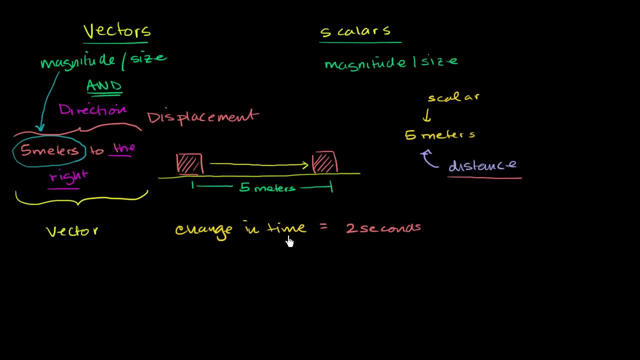 I guess, because there's only one direction for time as far as we know, or at least in that, what we're in, what we're going to deal with for the simple physics. So what is so? what's a measure of how fast this thing moved? 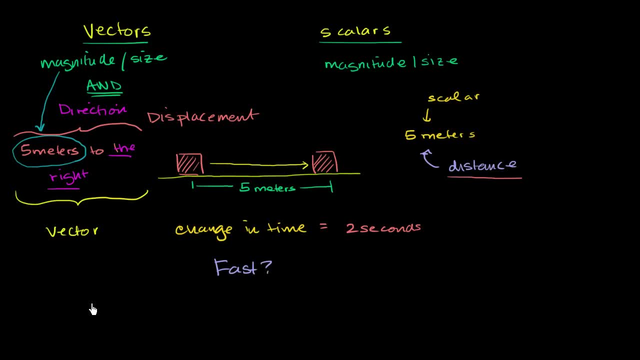 So how fast did this thing move? So we could say it moved 5 meters in 2 seconds. So let me write this down: So it moved 5 meters. it moved 5 meters per 2 seconds, per 2 seconds. 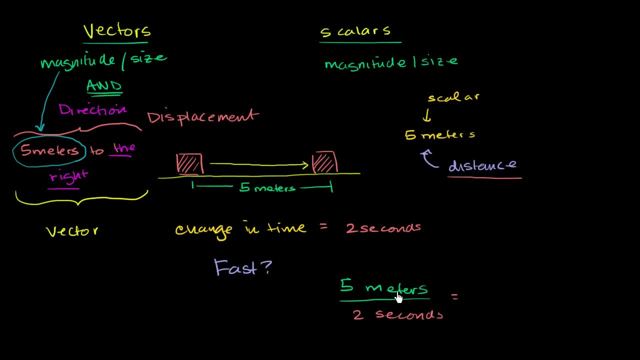 Or we could write this as 5 halves of a meter per second, Or 5 divided by 2. is what? 5 divided by 2 is: 2.5 meters per second. Meters per second. This right here is just the 5 divided by 2.. 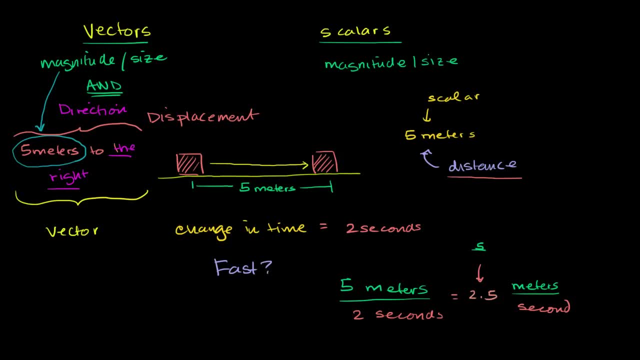 Let me make that clear That, right, there is just the 5 divided by the 2.. So my question to you, this 2.5 meters per second tells you how how far it traveled in a certain amount of time. Is this a vector or a scalar quantity? 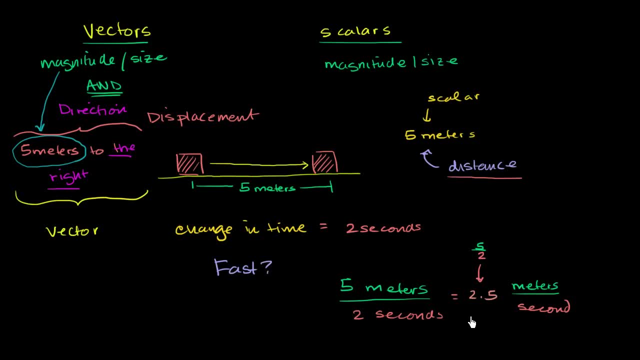 It is telling you how fast it went, but is it giving you just a, a size of this, of how fast it went, Or is it also giving you direction? Well, I don't see any direction here, So this is a scalar quantity. 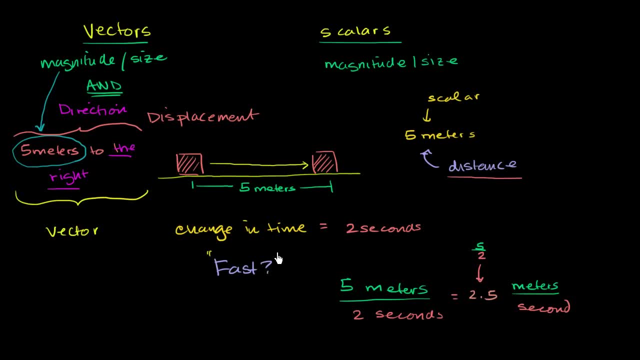 And the scalar quantity for how fast something is going. for how fast something is going is speed. So we could say that the speed of the brick is 2.5 meters per second. Now, if we do the same calculation, we say it went 2,. 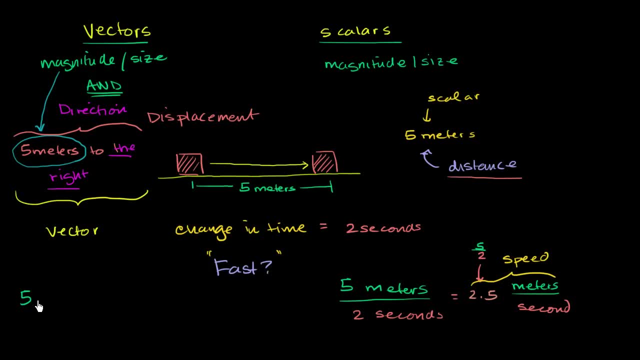 if we say it went 5, meters, 5, I'll just write m for meters, 5 meters to the right in 2 seconds. in 2 seconds, then what do we get? We get 2.5, once again. 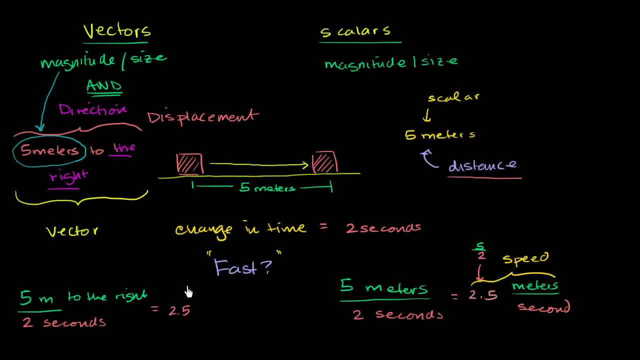 2.5 meters per second. I'll just abbreviate them as meters per second. meters per second to the right, to the right. So is this a vector or a scalar quantity? I'm telling you the the magnitude of the speed. 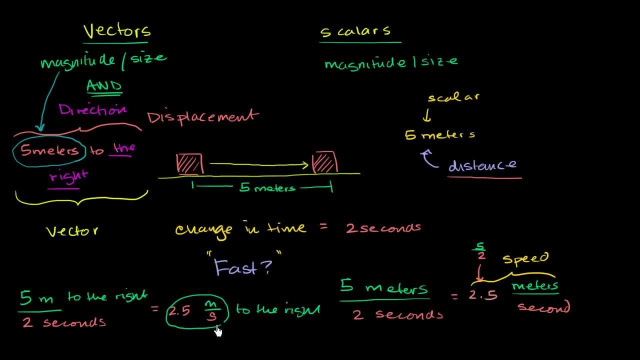 That's right here. This is the magnitude, 2.5 meters per second, And I'm also telling you the direction to the right. So this is a vector quantity. This is a vector quantity And when you specify both the speed,